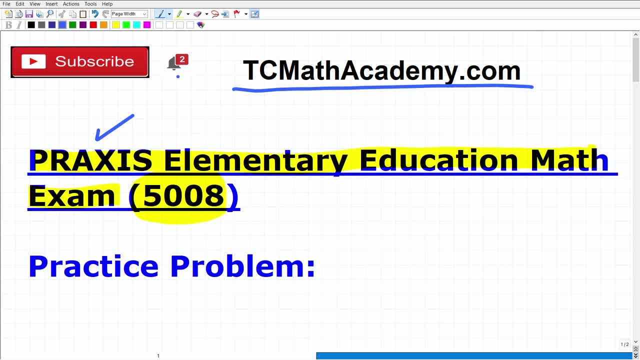 Okay, You're really going to have to know a lot of algebra, geometry and a lot of other stuff as well, but it's nothing that you can't do. You- certainly you know at this point in your life um have already have the educational background to be successful, but you're going to have to get really re-immersed in mathematics to be fully prepared for this particular exam. 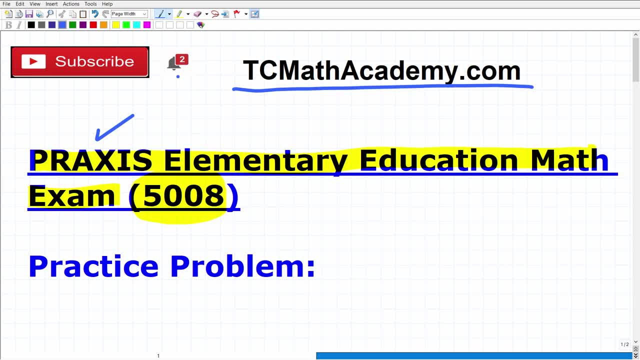 Now, uh, I have an outstanding test prep course for this practice exam. You can find a link to that in the description of this video, So if you're looking for a great way to prepare my course, we'll definitely help you out. 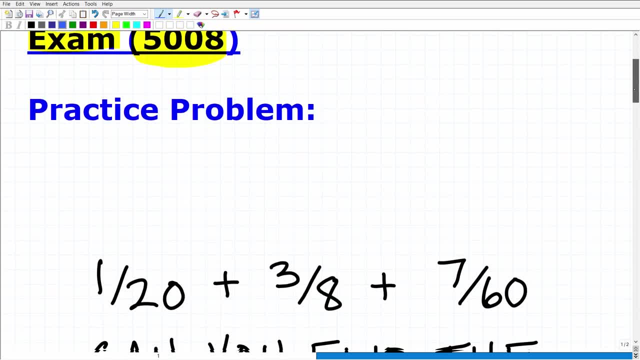 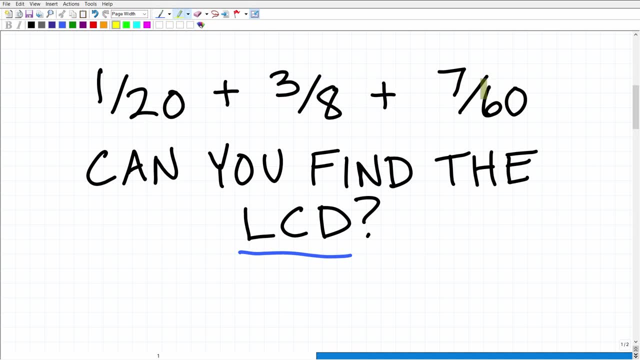 Okay, So let's go ahead and get into this problem. So here we have three fractions. The question is not to find the sum. I'm not interested in adding these fractions up, I just simply want to know what is the lowest common denominator. 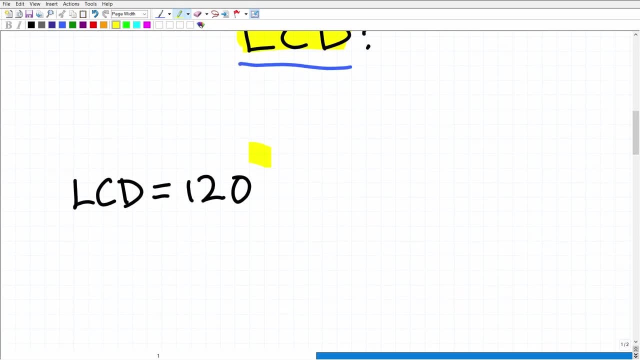 All right, Let's go take a look at the answer. The answer is one: 20.. Okay, So that is the answer. Now, if you got the answer right, that is fantastic. So that's kind of like that, Okay. 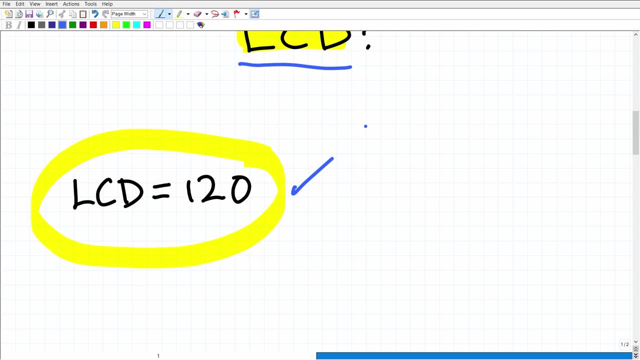 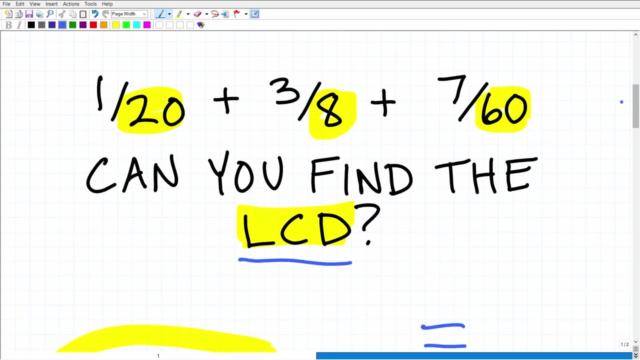 Kind of like one part of the question. The next part is: how do you find the LCD? And these values here are not that difficult. You know, I could certainly have made this problem much more challenging. I could have put like, say, 208,, uh 88 and maybe 609, or something like that. 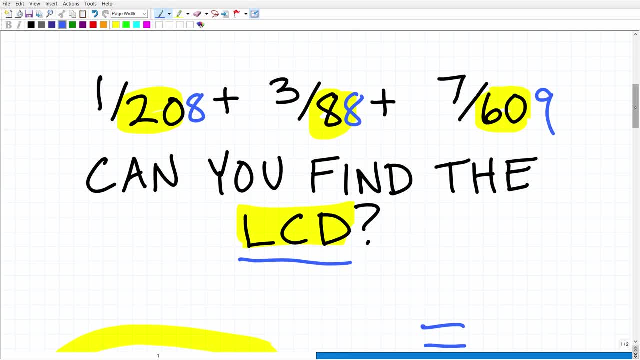 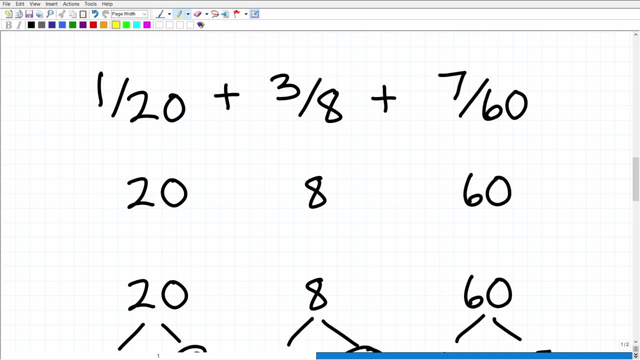 This would have been much, much more difficult problem, but nevertheless, you know the procedure doesn't change, So let's go and talk about how to do this problem. All right, So the first thing is, when you're talking about finding the lowest common denominator, we need to just, uh, take into account the denominators of the respective fractions that we're looking to add or subtract. 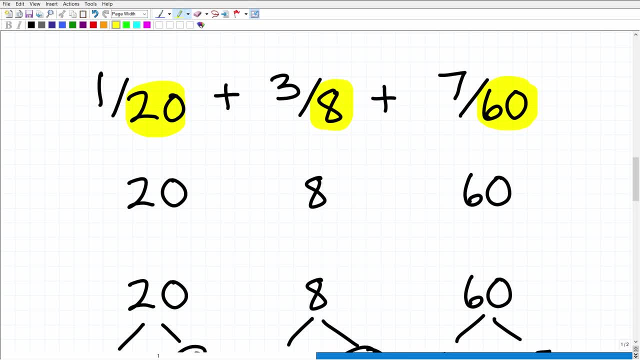 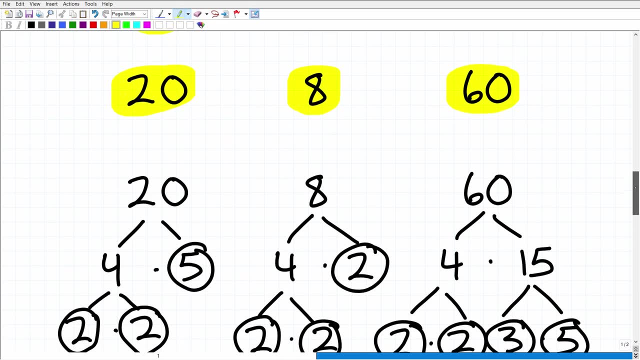 So here we're talking about 28 and 60. All right, So we got to take these three numbers and what you want to do is prime factor each of these numbers, and a great way to factor any number is to use a factor tree. 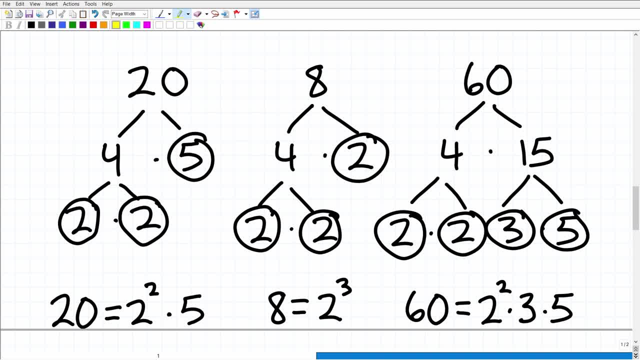 So let's go to Take a look at this uh work right here. Of course you could say I've already done the work. So here's 20, here's eight and here's 60.. Let's uh focus in here on a 20 year. 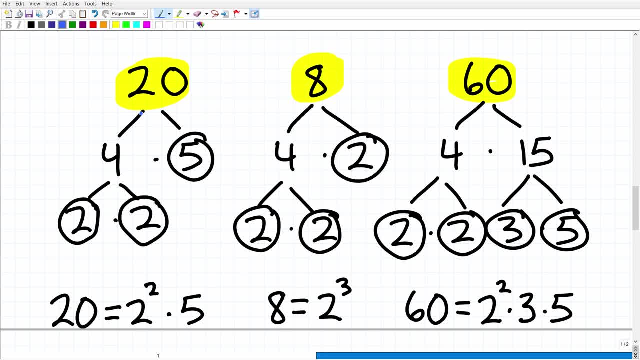 Okay, So we're going to factor 20.. Now the factors are 20.. There's any number of different ways you can approach this. You can be like, oh, this is uh, uh, two times 10.. That's fine. 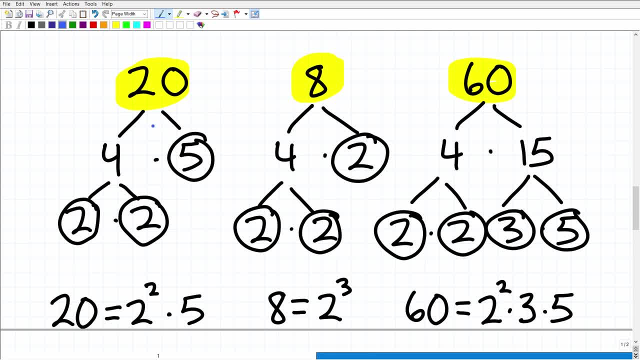 Uh, you just want to find a pair of factors for 20, but you're looking to prime factor. So let's, uh, take two numbers that we know. when we multiply them, Yeah, Together we get back to 20.. 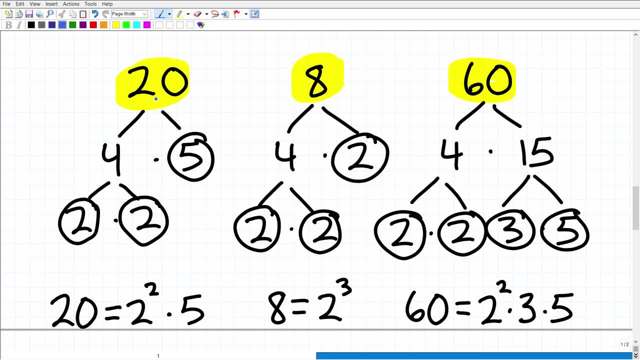 So that'd be four and five. Now, these are the factors of 20.. So I'm asking myself: okay, or either one of these factors, a prime number. if it's prime, I'm going to circle it. So in this case, five is prime. 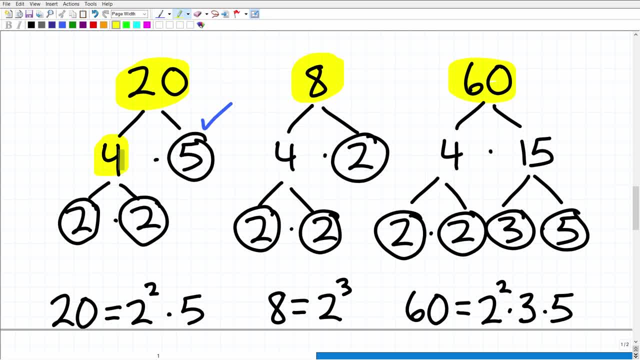 So I'll circle that And I see four is not prime. I could continue to factor four into two times two, which of course two and two are prime. Okay, So two, two and five are my prime factors of 20. Okay. 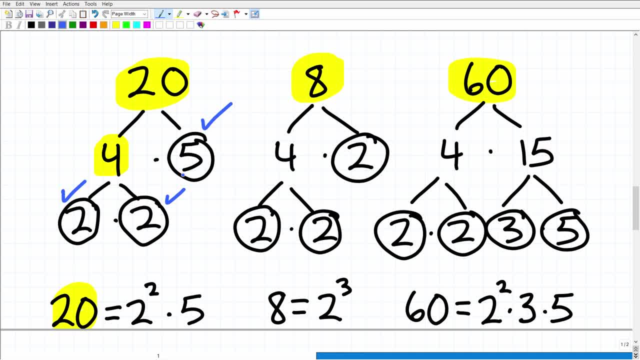 So 20 is equal to two times two times five, Uh, so you always want to um, write, uh, any repeating um, uh values that are being multiplied together like this: two times two, as powers. You'll see why here, in a second. 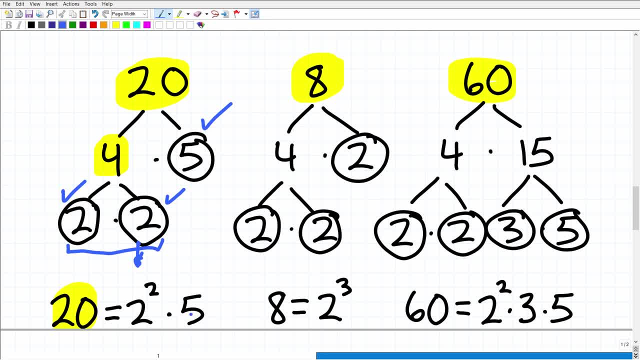 So 20 is really equal to two squared times five. Okay, So let's take a look at eight. So eight is four times two. two is prime. I can continue to factor four, So that's two times two. So eight is equal to two times two times two. 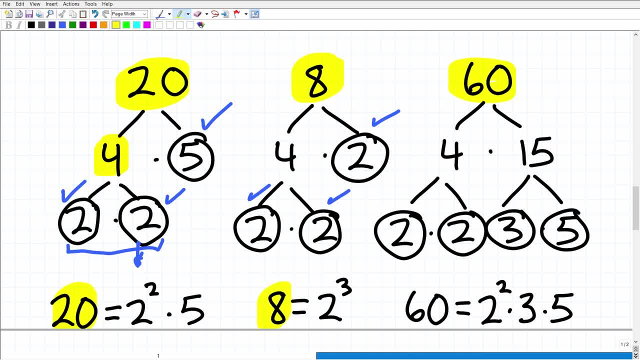 And of course two is prime, And of course I want to again again express that as a power. two times two times two, We can write as two cubed And you can see the work here for 60.. Uh, even if you want two times 30,, don't worry about it. 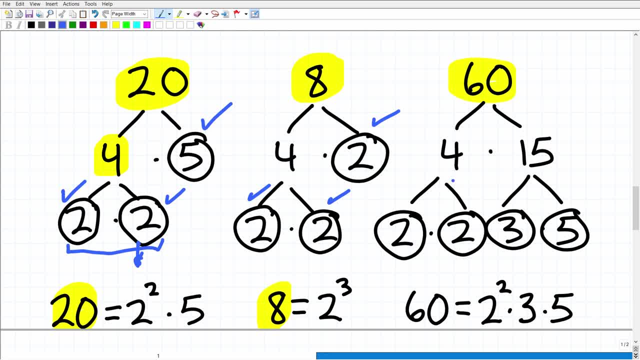 When it comes to a factor tree, you'll, uh long as you continue to um factor all the factors down to the prime factors, you'll still get the right answer. So 60 is going to be equal to two squared times three times five. 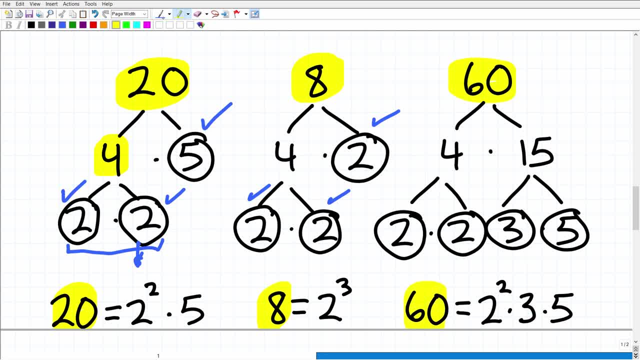 And you can see the work right there. Okay, So what do we do next? Well, this is the Step one. so the first step you know, in terms of instructing a student would be like: okay, let's, you know, you have to learn how to prime factor right. 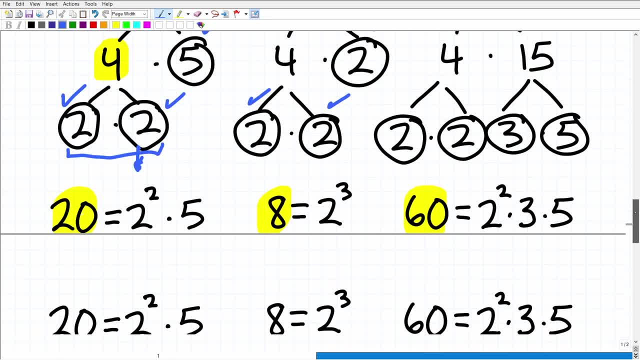 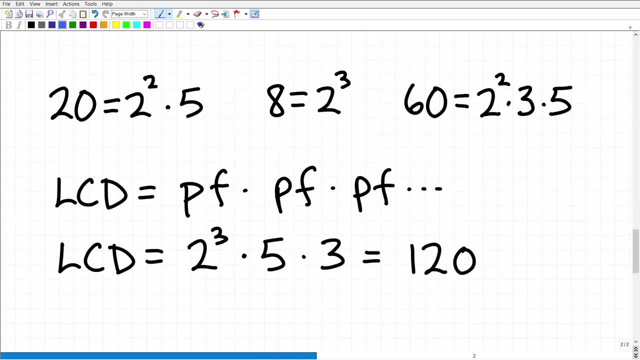 So that's the first thing. The second thing you need to do is have a um, a kind of a formula to actually find the LCD. Now there are easier, more um, kind of intuitive ways when we're talking about real simple. 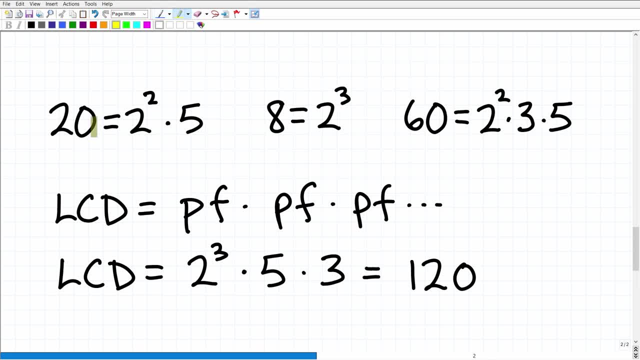 simple values about the lowest common denominators, But the kind of the procedure I'm talking about here is something that will carry on for much more challenging arithmetic problems and algebra- Okay, It's actually the same procedure, uh, to find the lowest common denominator. 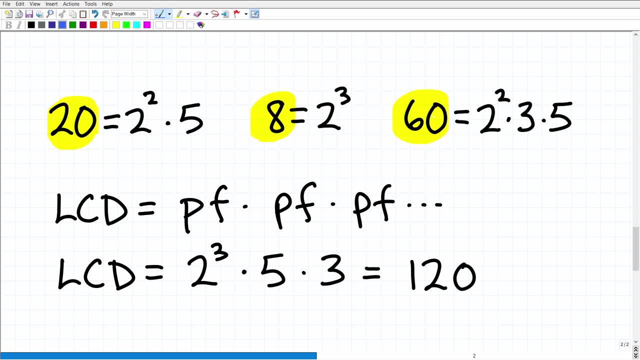 When you have algebraic uh expressions, rational expressions, we call them All right. So the lowest common denominator is going to be equal to the product. Okay, Of all the various prime factors, Okay, So we're going to scan through all of our prime factors here of the denominators and we're going to 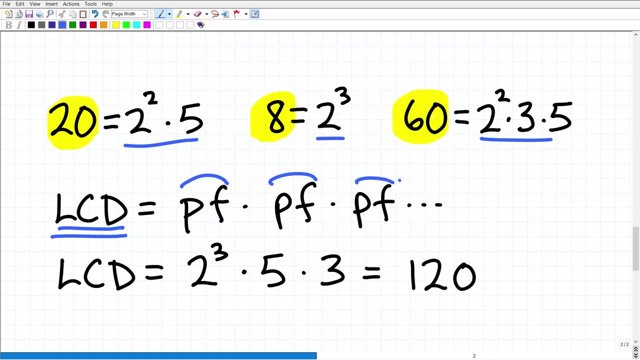 take each unique prime factor And we're going to Multiply them together. All right, So we're going to have to have each prime factor represented uh into the LCD and then we're going to multiply them together and we'll actually get the right answer. 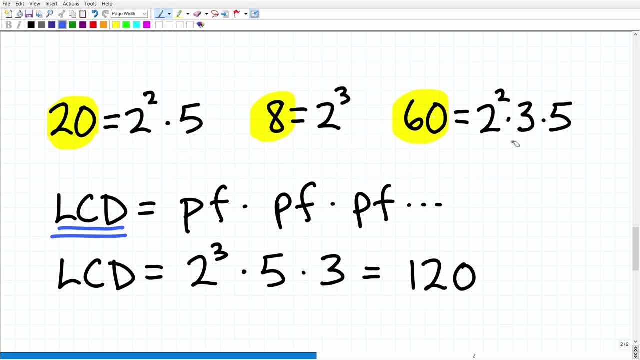 Okay. So now let's take a look at what we have. Let's start off with the- um, most challenging part of this, And that is, uh, the dealing with the twos here. Okay, So here I have two squared here. 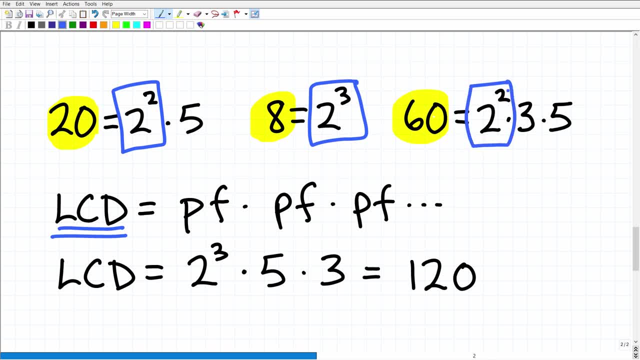 I have two cubed in here. I have two squared. right now I'm looking at this. I'm like, Okay, Do I need to have a two squared malt you know in my prime factor? Uh, do I also need to have a two cubed and another two squared? 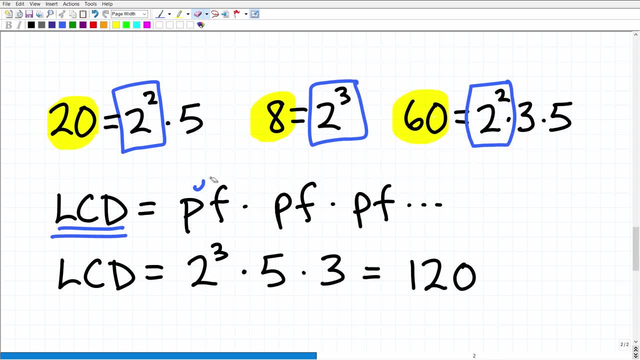 No, we just need to represent uh two, the number two. but which number two? the two squared, or the two cubed or the two squared? Well, the way it goes is, you need to identify the highest power, uh, of these various um, uh. 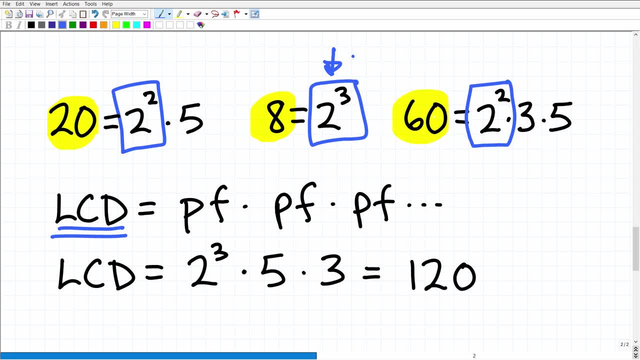 bases that you have. So if you have two squared and two cubed, you need to have The two cubed. represent, uh, that power of two. All right, So hopefully I said that in a non confusing way. but here our first prime factor is going. 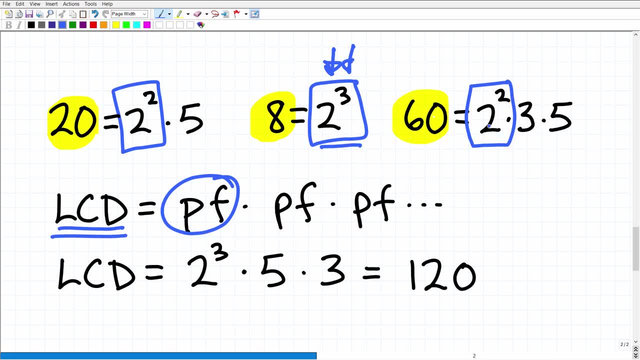 to be two cubed. We don't need to have all the twos represented. uh, just one. two. which power of two? the highest power that you have. Okay, So that's going to be two cubed, All right.